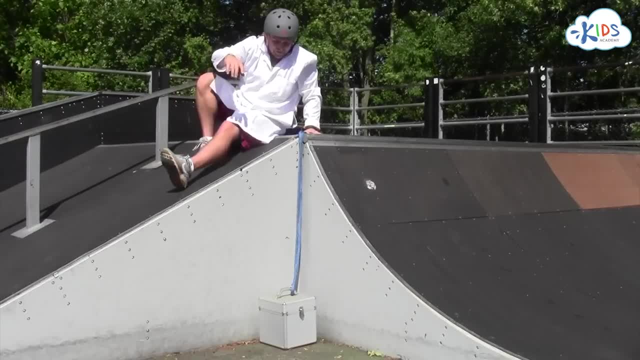 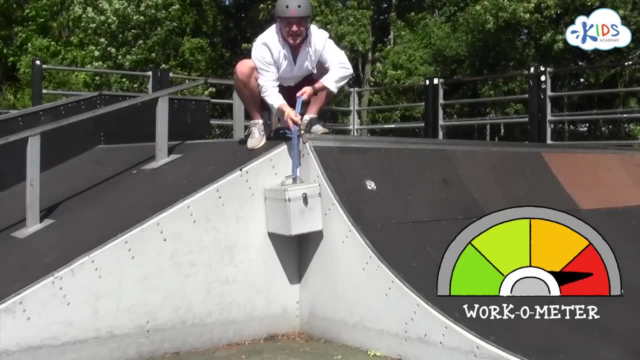 balls- big heavy balls- and try and lift them straight up. Let's see how that goes. Now. this is a big heavy crate. You can see, it's taking a lot of effort and a lot of work for me to get it up here. 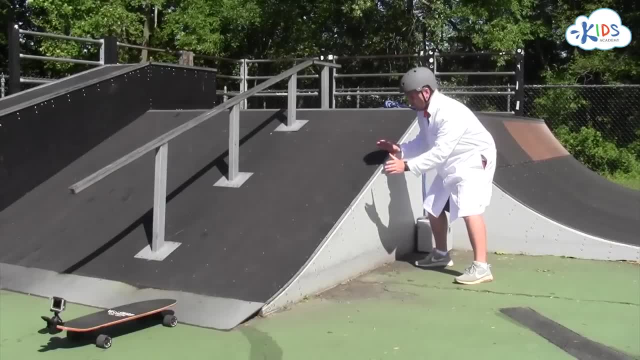 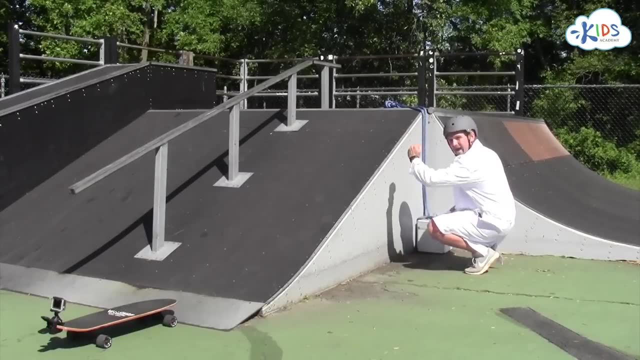 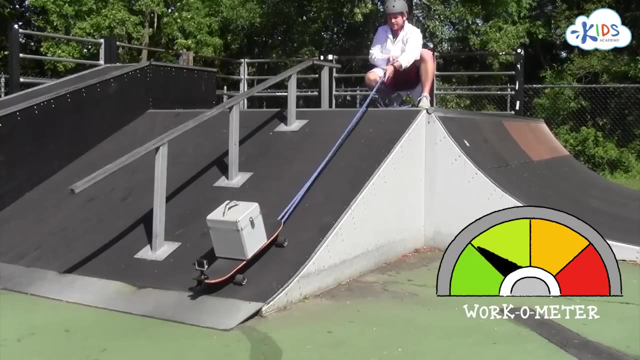 Too much. There's got to be a better way. I have here a ramp. Now. this ramp can still get me from the ground to the top, But just at a different angle. I'm going to use science and my brain to make it easier. 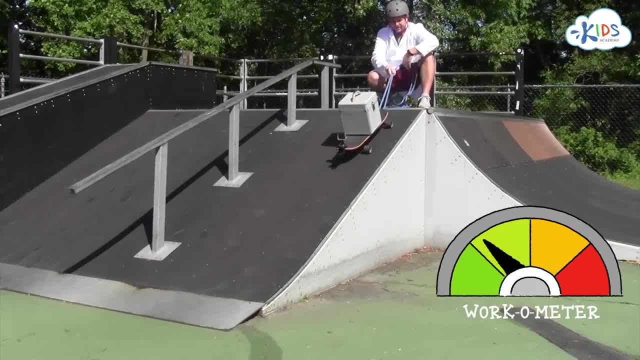 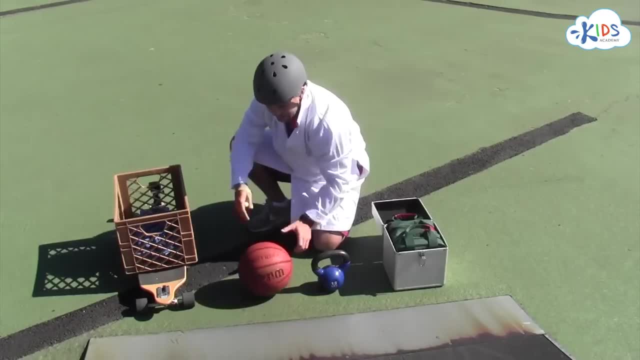 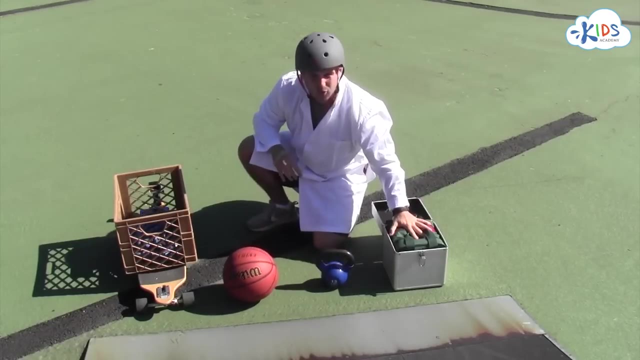 Now I barely even need to pull and I can get the crate all the way to the top. We've got a bit of an experiment set up. We have a basketball, we have a 15 pound kettle bell and we have a whole box full of bocce. 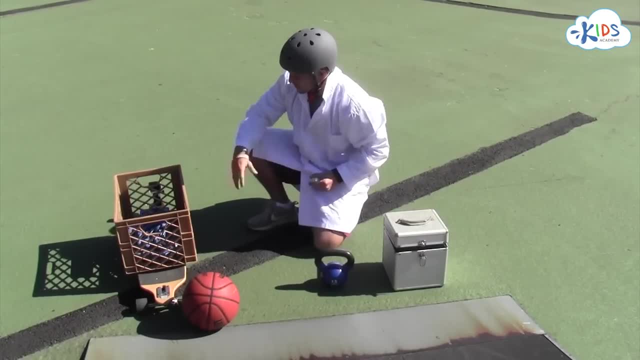 balls. So what we're going to do is we're going to put each one of these objects into our skateboard crate of science and we're going to roll it down this ring. Then we're going to find out how far it goes and we're going to mark the distance with 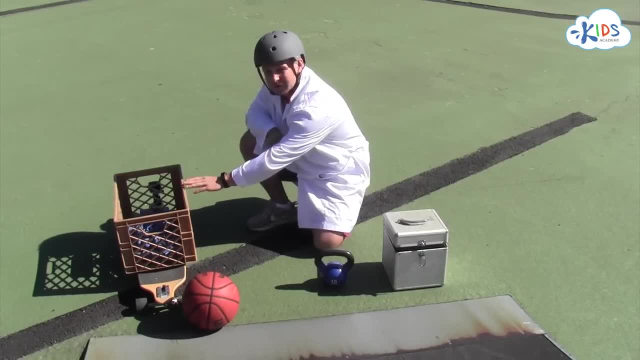 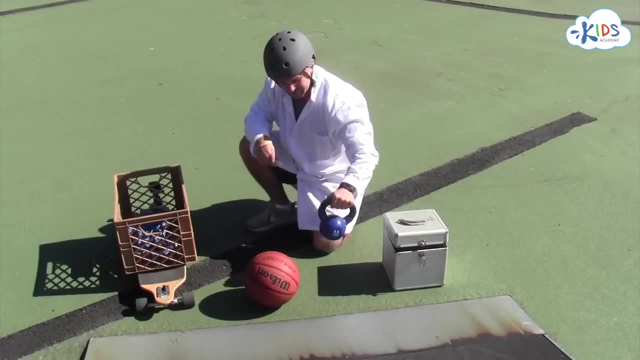 each piece of chalk. So first we'll test the skateboard with just the crate and nothing inside it, Then we'll test it with the basketball, then test it with our 15 pound weight and then test it with our bocce balls. 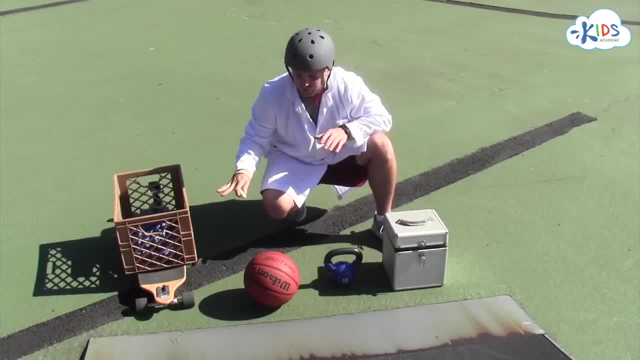 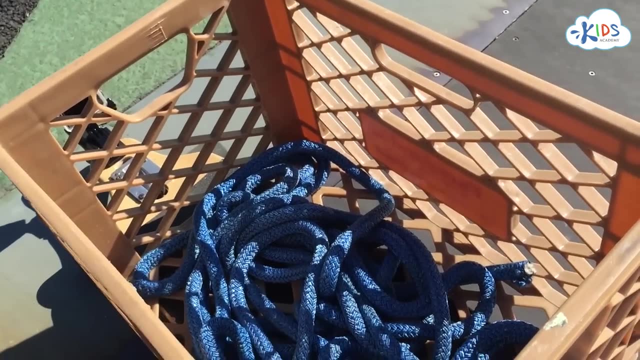 Which item? Or the empty skateboard, Which item? Which item do you think is going to travel the farthest after rolling down a ramp? First up is our empty crate. You can see there's a rope in there. The rope is actually tying the crate down so that we don't lose it. 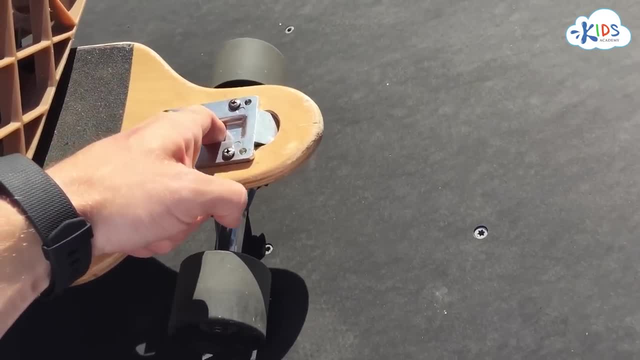 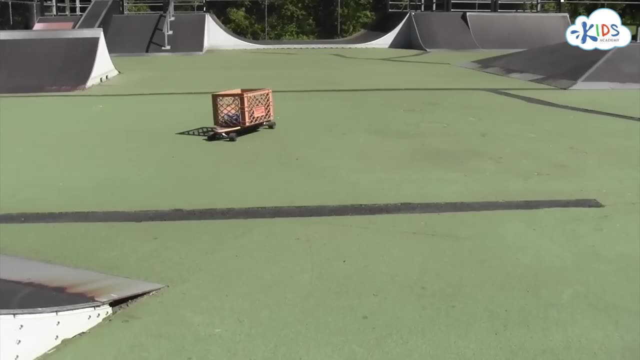 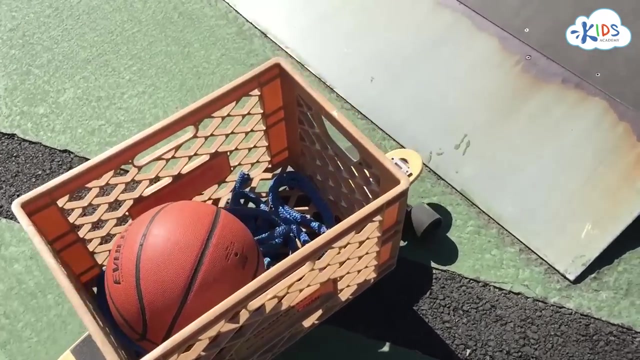 I made two lines here so I can see where the wheels go to each time, so that each object is released from the same distance. Okay, Now let's load up our basketball and see how far this takes us. I'm going to pull it back to the same place. 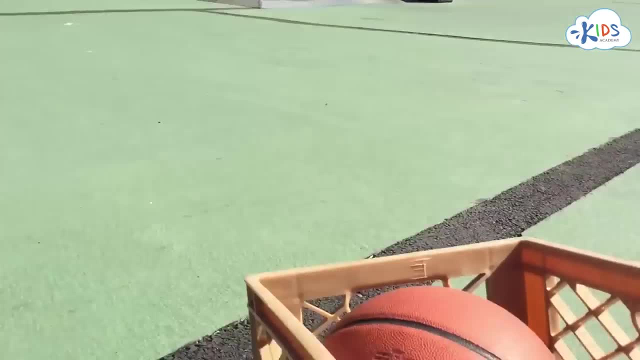 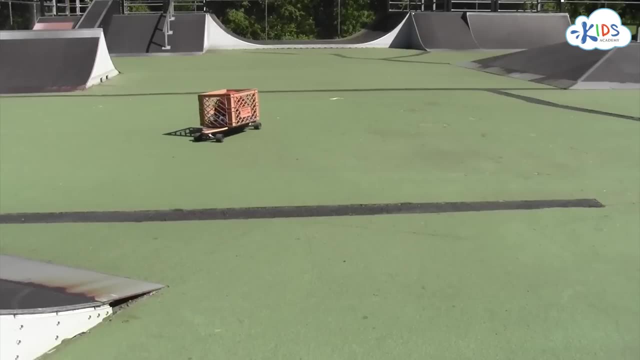 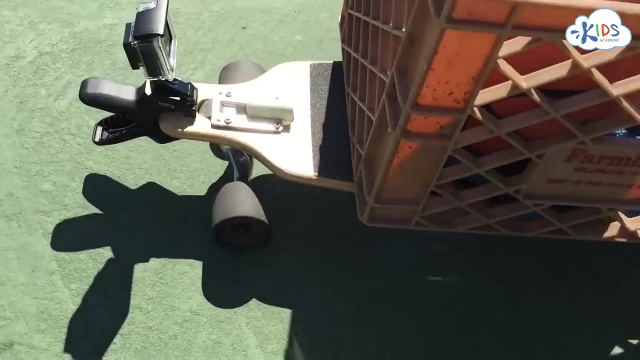 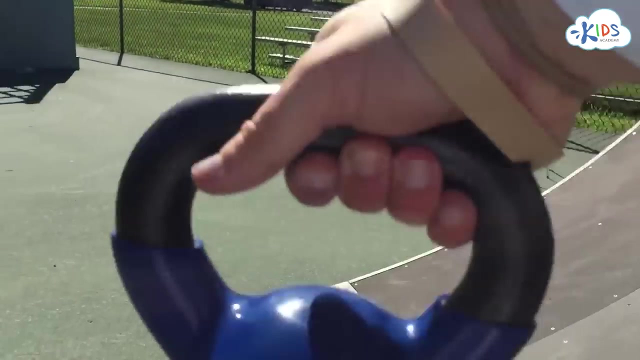 I have my skateboard aiming the same direction. Basketball is in and let's send it on. Okay, Cool, All right now. the last basketball, and not weighing very much, almost made it to our empty, but came up just a little bit short. now we're gonna load up our 15 pound weight. 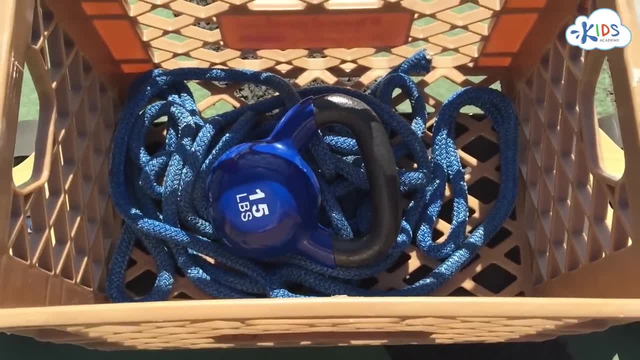 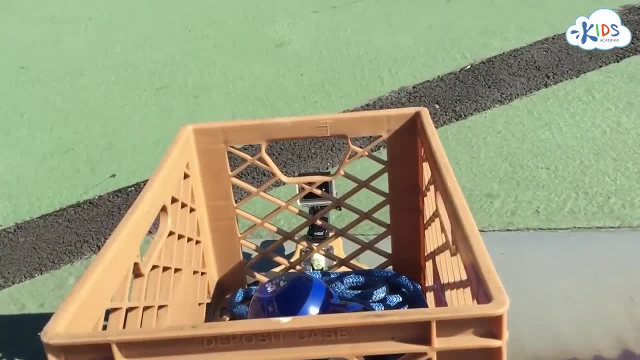 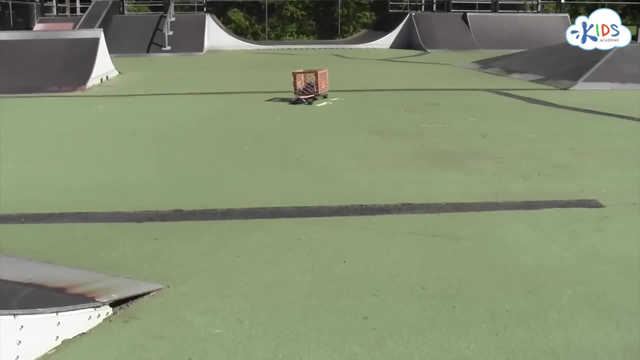 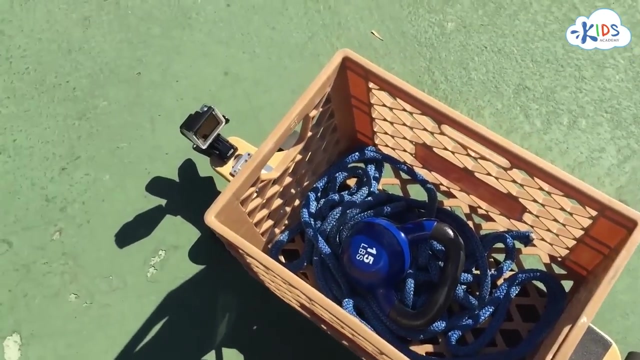 now, this is significantly heavier than the basketball. do you think it'll go farther, or not as far as our basketball and our empty crate? let's send it off. there's the basketball. the empty crate and our 15 pound weight has made it all the way here. let's make a mark there. we're at the 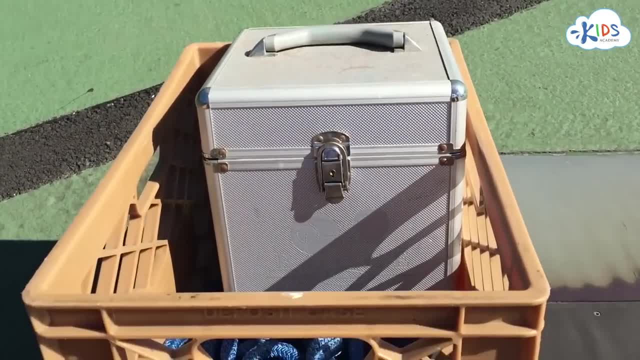 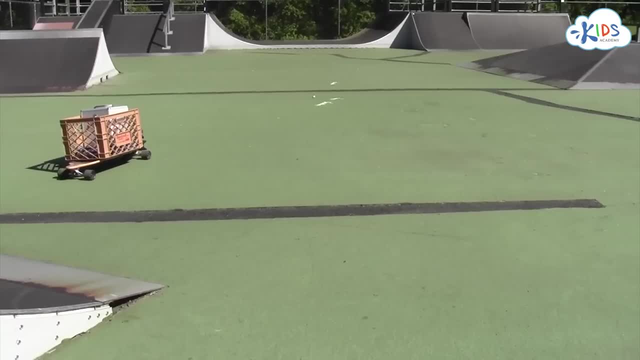 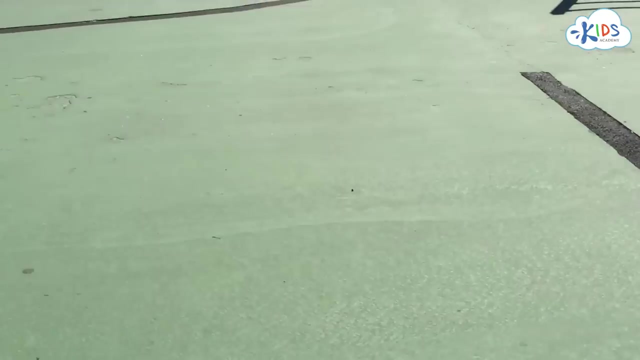 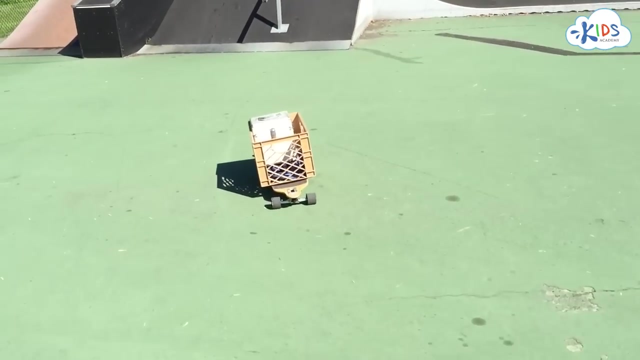 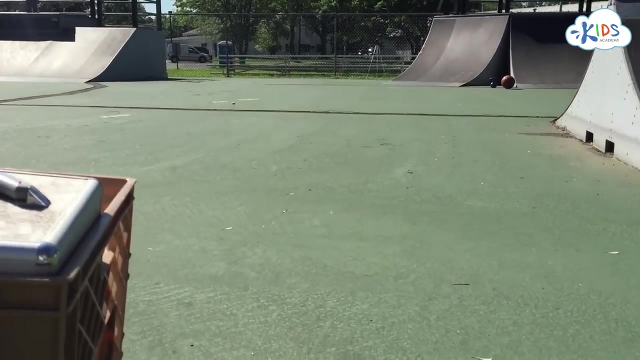 drop line. now how far do you think this one's gonna go? let's send it off. that last one traveled significantly farther. there's the basketball, there's the empty crate, there's the 15 pounds, and our bocce ball made it all the way down here, it seems. the heavier the 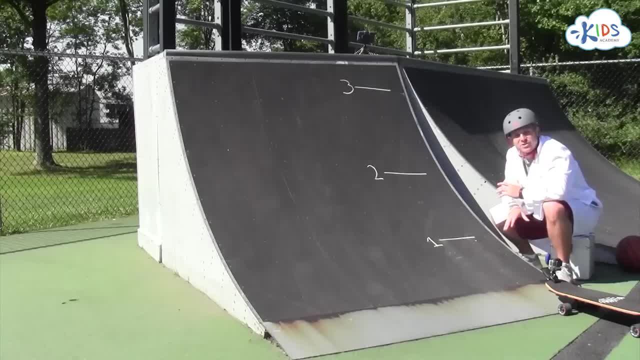 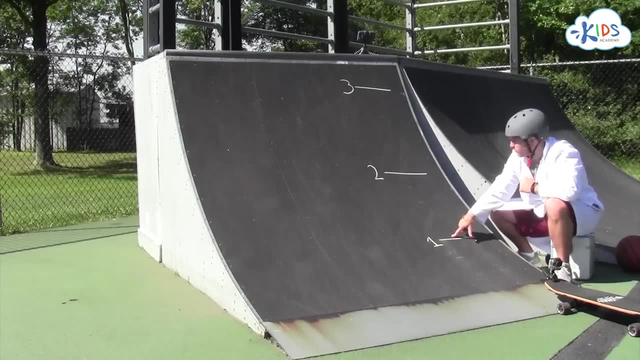 object on the skateboard the farther it traveled. now let's try launching our skateboard from different heights on our ramp. we have launched number one, where the back wheels will be at this line. we have launched number two, where we'll pull the back wheels all the way up to here, and then we have launched three.